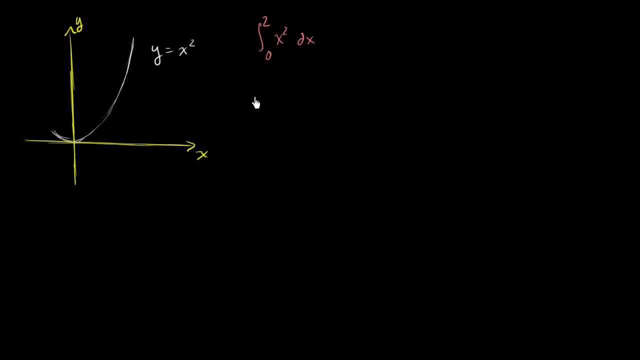 and 2 of x squared dx, what does that represent? Let's look at our end points. So this is x is equal to 0. Let's say that this right over here is x is equal to 2. 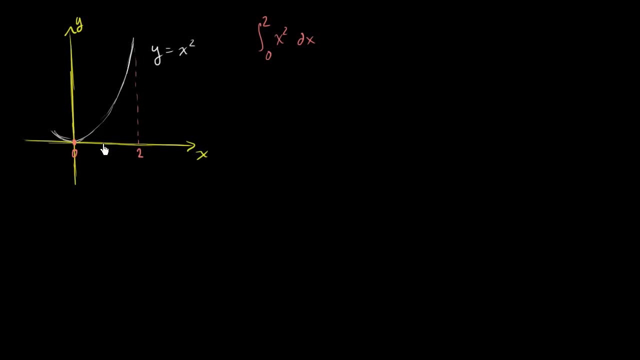 What we're doing is for each x, we're finding a little dx around it. So this right over here is a little dx. And we're multiplying that dx times our function, times x squared. So what we're doing is we're multiplying this width times this height right over here. The height right over here is x squared. And we're getting the area of this little rectangle. 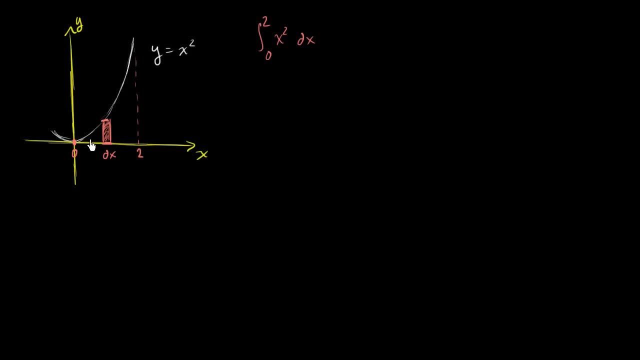 And the integral sign is literally the sum of all of these rectangles for all of the x's between x is equal to 0 and x is equal to 2. 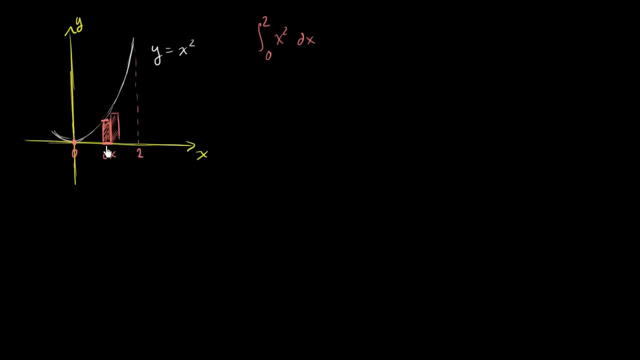 But the limit of that, as these dx's get smaller and smaller and smaller, get infinitely small, with not being equal to 0, and we have an infinite number of them. 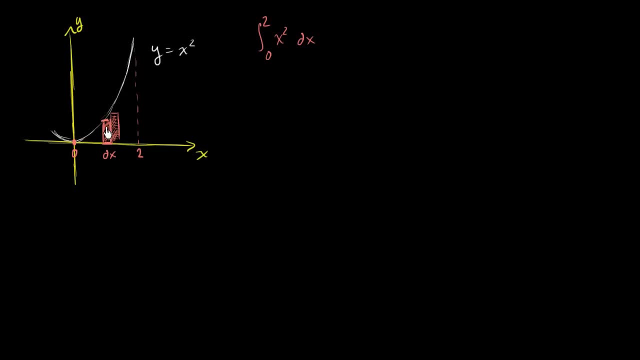 That's the whole power of the definite integral. And so you can imagine as these dx's get smaller and smaller and smaller, these rectangles get narrower and narrower and narrower. 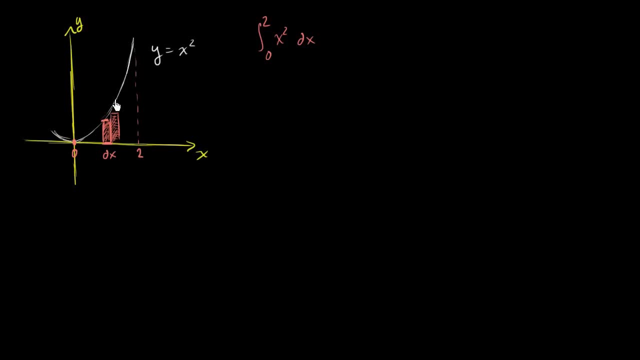 And we have more of them. We are getting a better and better approximation of the area under the curve until, at the limit, we are getting the area under the curve. 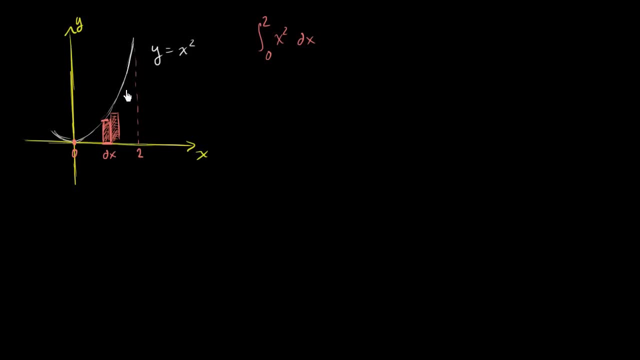 Now we're going to apply that same idea, not to find the area under this curve, but to find the volume if we were to rotate this curve around the x-axis. So this is going to stretch our powers of visualization here. 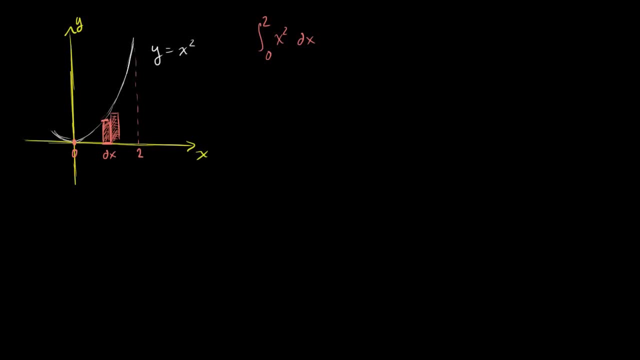 So let's think about what happens when we rotate this thing around the x-axis. 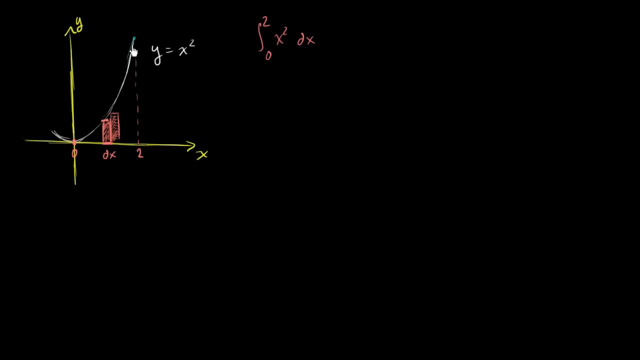 So let's rotate it. And say we're looking at it a little bit from the right. So we get kind of a base that looks something like this. 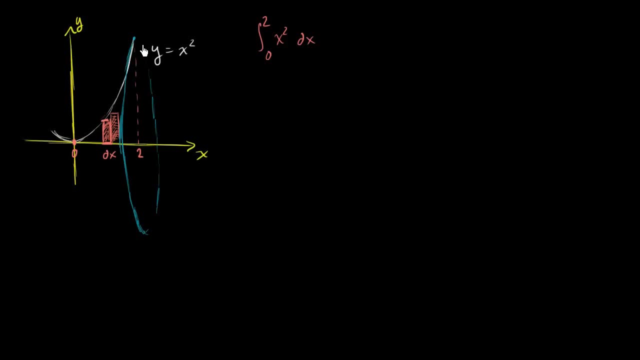 So this is my best attempt to draw it. So you have a base that looks something like that. And then the rest of the function, 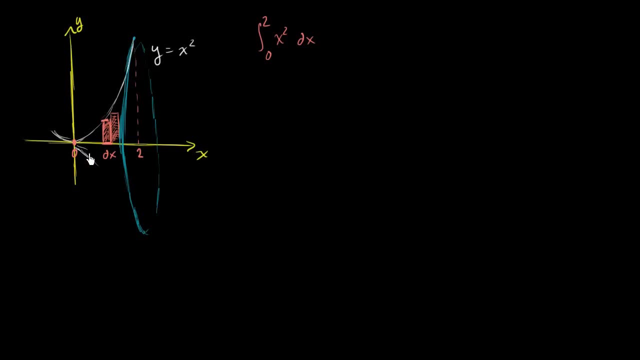 it looks kind of like, if we just think about it between 0 and 2, it looks like one of those pieces from, if you ever played the game, Sorry. 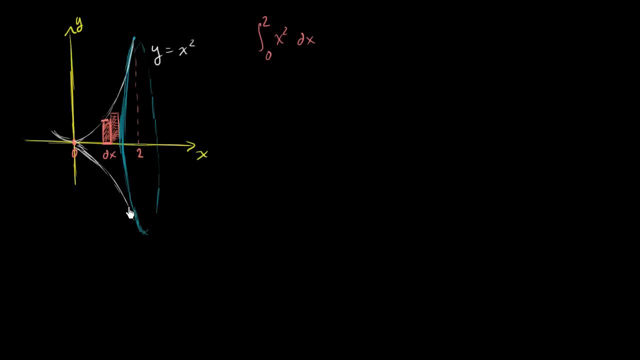 Or it looks like a little bit of a weird hat. 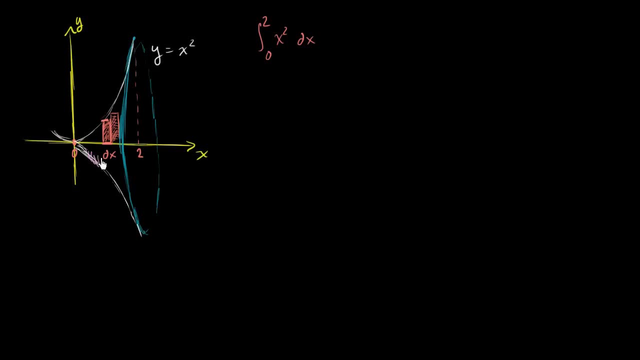 So it looks like this. And let me shade it in a little bit. Shade it in a little bit, so it looks something like that. 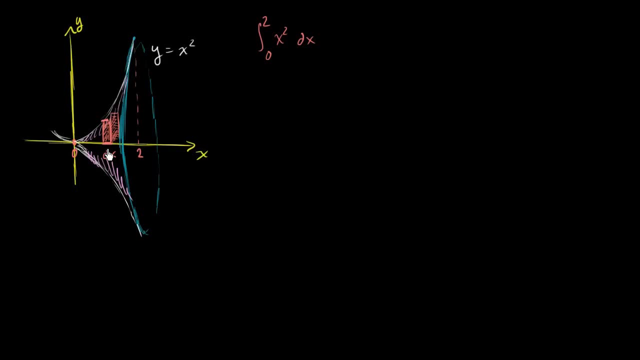 And just so that we're making sure we can visualize this thing that's being rotated, and we care about the entire volume of the thing, let me draw it from a few different angles. So if I drew it from the top, it would look something like this. It would become a little more obvious. 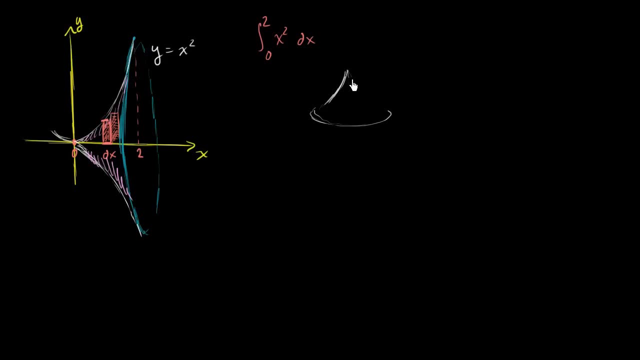 It would look something like a hat. Point up like this, and it goes down like that. It would look something like that. 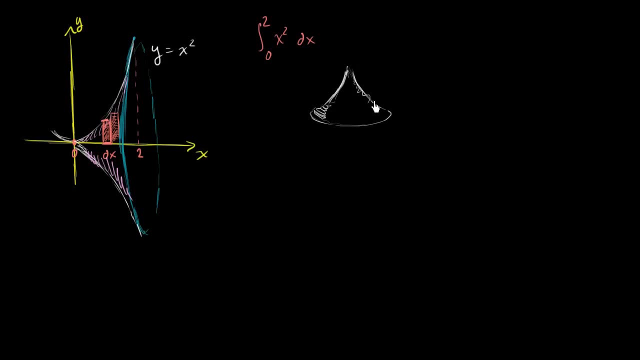 So we're not seeing, in this angle, we're not seeing the bottom of it. 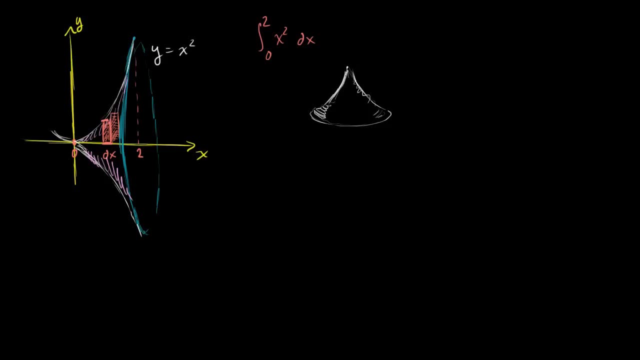 And just to orient yourself, if you were to orient yourself, the axes, in this case, look like this. So this is the y-axis. 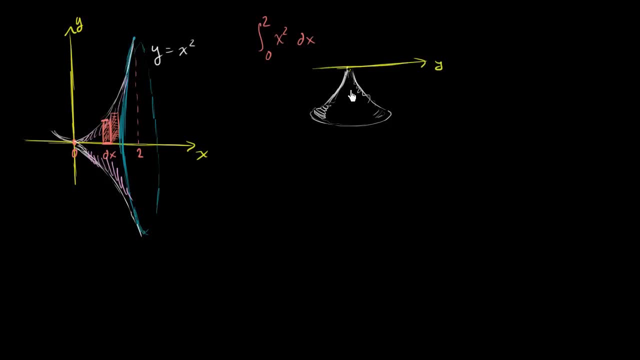 That is the y-axis. And then the x-axis goes right inside of this thing, and then pops out the other side. And if this thing was transparent, then you could see the back side. It would look something like that. The x-axis, if you could see through it, would pop the base right over there, would go right through the base right over there, and then come out on the other side. 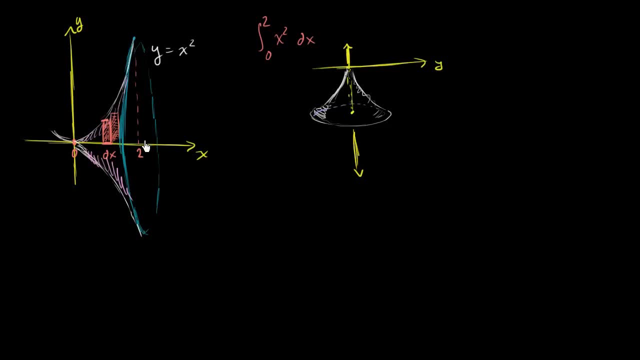 So this is one orientation for the same thing. You could visualize it from different angles. 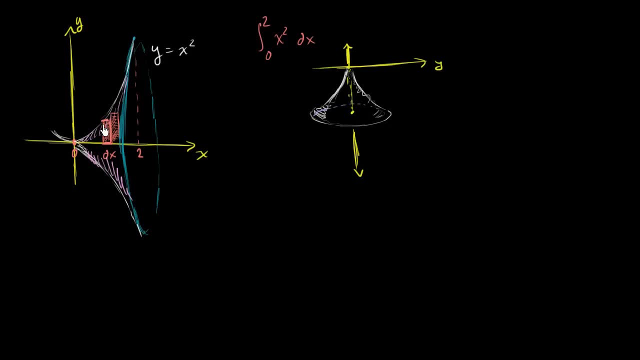 So let's think about how we can take the volume of it. Well, instead of thinking about the area of each of these rectangles, what happens if we rotate each of these rectangles around the x-axis? 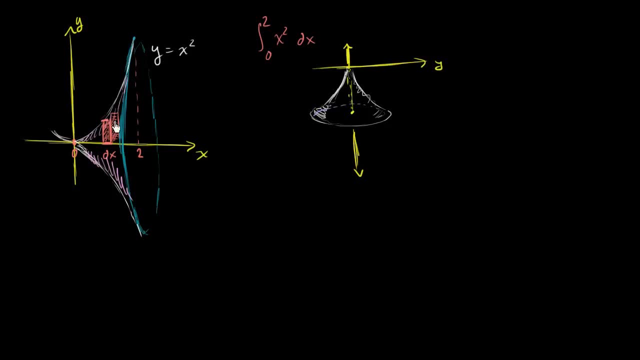 So let's do it. So let's take each of these. Let's say you have this dx right over here, and you rotate it around. 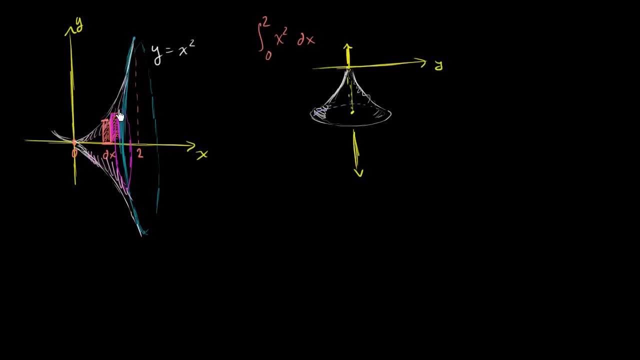 Around the x-axis. So if you were to rotate this thing around the x-axis, so I'm trying my best to. Around the x-axis, you rotate it. 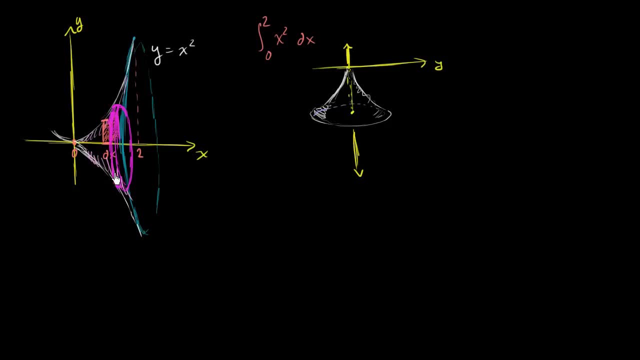 What do you end up with? What do you end up with? Well, you get something that looks kind of like a coin, 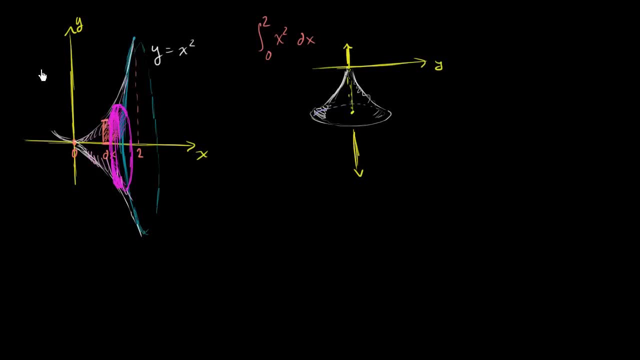 like a disk, like a quarter of some kind. Let me draw it out here. 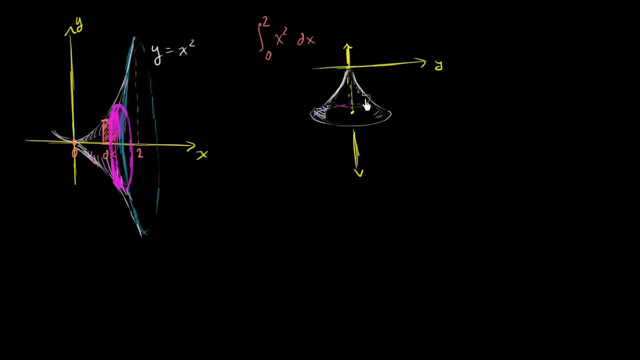 So if you were to do that same disk out here, it would look something like this. 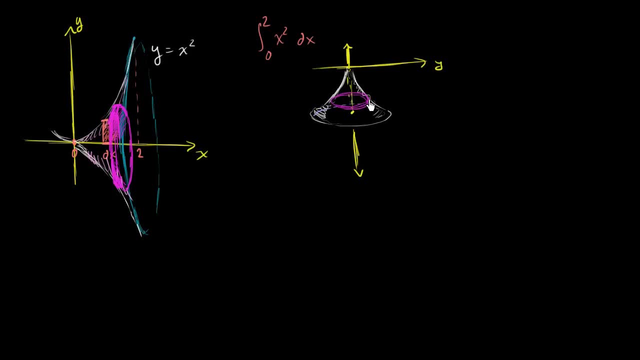 It would look something like this, and it has a depth of. 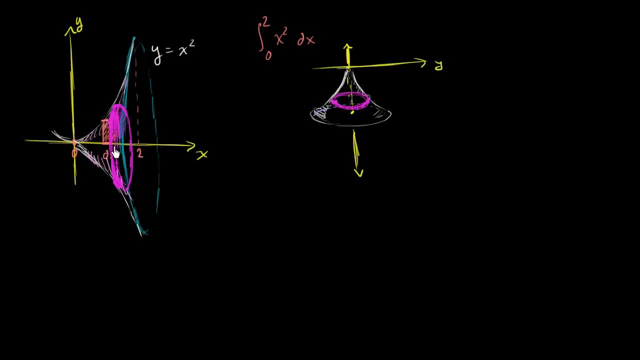 dx. So how can we find the volume of that disk? Let me redraw it out here, too. 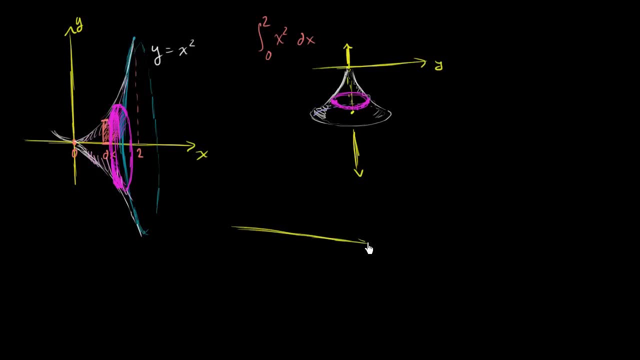 It's really important to visualize this stuff properly. So this is my x-axis. 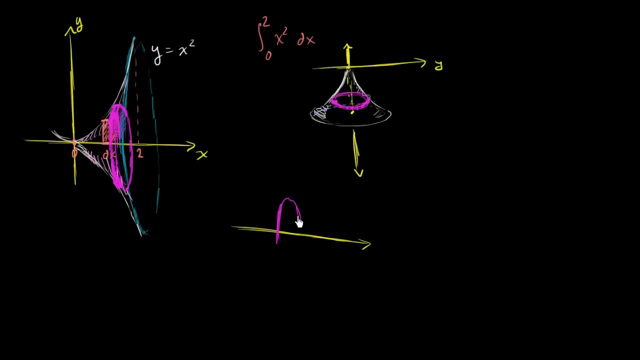 My disk looks something like this. My best attempt. The x-axis hits it right over there, comes out of the center, and then this is the surface of my disk, and then this right over here. 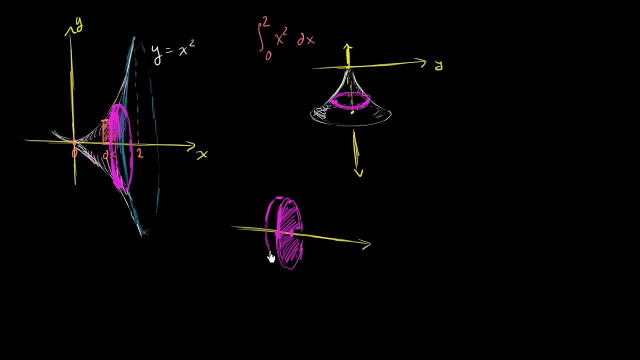 Here is my depth, dx. So that looks pretty good. And then let me just shade it in a little bit to give you a little bit of the depth. 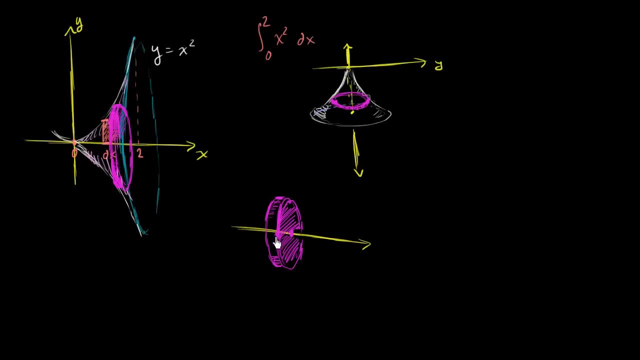 So how can we find the volume of this? Well, like any disk or cylinder, you just have to think about what the area of this face is, and then multiply it times the depth. So what's the area of this face? Well, we know that the area of a circle is equal to pi r squared. So if we know the radius of this face, we can figure out the area of the face. All right. All right. So what's the area of this face? 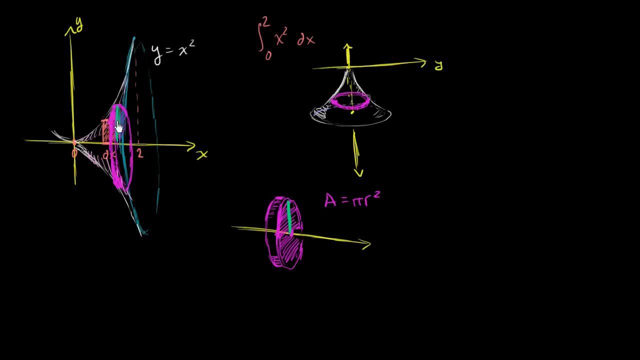 Well, what's the radius? Well, the radius is just the height of that original rectangle. And for any x, the height over here is going to be equal to f of x. And in this case, f of x is x squared. So over here, our radius is equal to x squared. 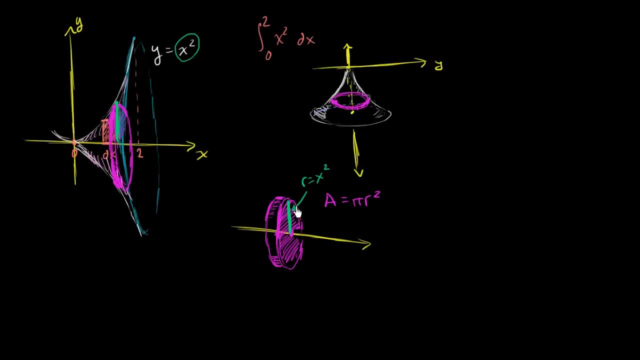 Radius is equal to x squared. So the area of the face for a particular x is going to be equal to pi times f of x squared. In this case. 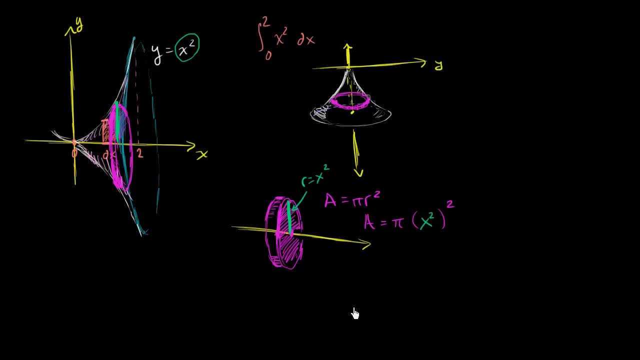 In this case, f of x is x squared. Now, what's our volume going to be? 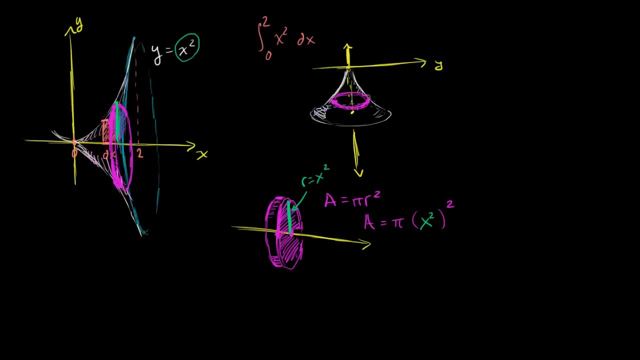 Well, our volume is going to be our area times the depth here. It's going to be that times the depth times dx. So the volume of this thing right over here, so the volume just of this coin, I guess you could call it, is going to be equal to, so my volume is going to be equal to, my area times dx, which is equal to pi times x squared squared. 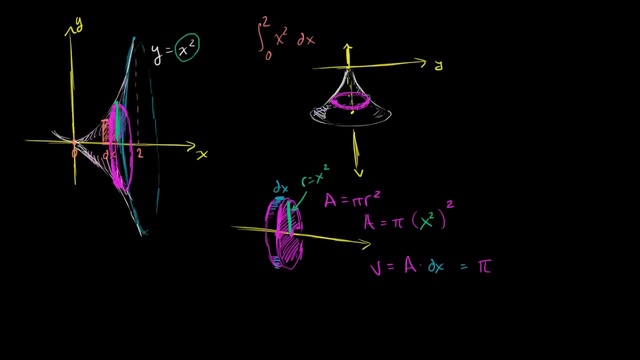 So it's equal to pi, x squared squared is x to the fourth, pi x to the fourth dx. 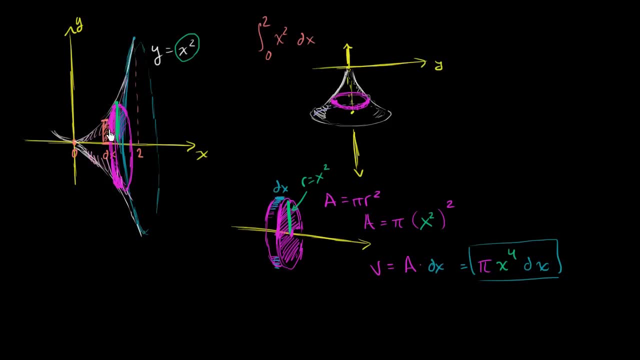 Now, this expression right over here, this gave us the volume just of one of those disks. But what we want is the volume of this entire hat, or this entire kind of. Bugle or cone looking, the front of a trumpet looking thing. So how could we do that? Well, the exact same technique. 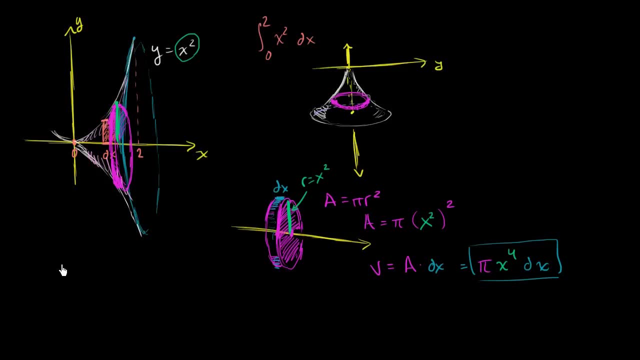 What happens if we were to take the sum of all of these things? So let's do that. Take the sum of all of these things. And I'll switch to one color. Pi times x to the fourth dx. We're going to take the sum of all of these things from x is equal to 0 to 2. Those are the boundaries that we started off with. I just defined them arbitrarily. We could do this really fast. We could do it for any two x values. 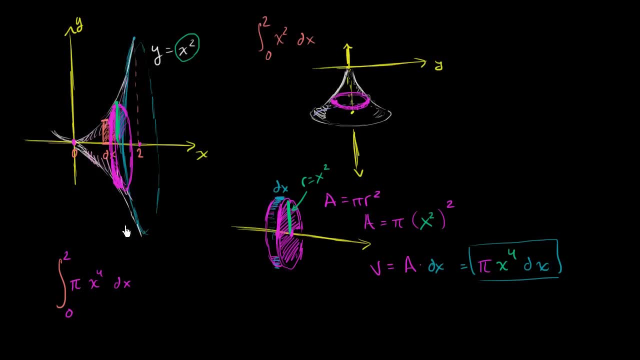 Between x is equal to 0 and x equals 2. And we're going to take the sum of all of these, 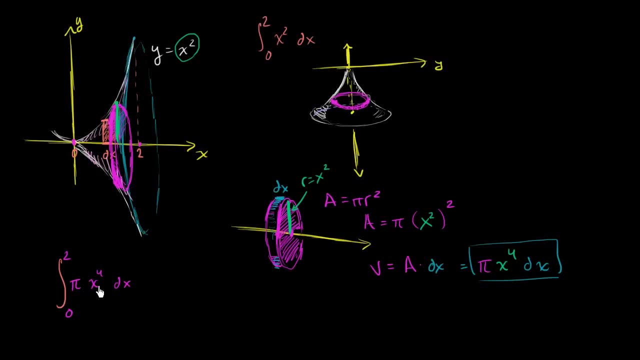 the volumes of all of these coins. But the limit, as the depths get smaller and smaller and smaller and we have more and more and more coins, at the limit, we're actually going to get the volume of our cone, or our bugle, or whatever we want to call it. 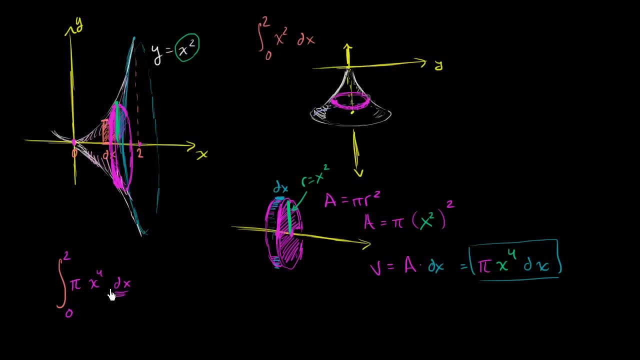 So if we just evaluate this definite integral, we have our volume. So let's see if we can do that. 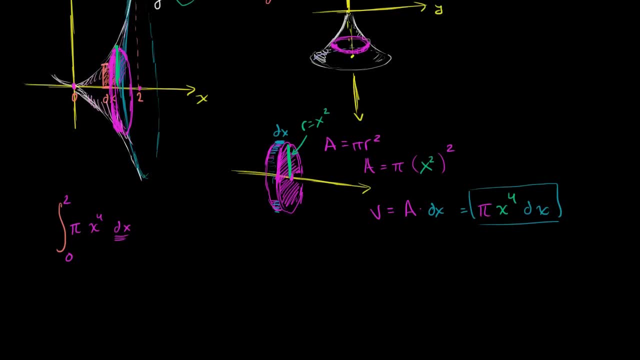 So this is, and now this is just taking a standard, definite integral. So this is going to be equal to, and I encourage you to try it out before I do it. So we could take the pi out. So it's going to be equal to pi times the integral from 0 to 2 of x to the fourth dx. I don't like that color. 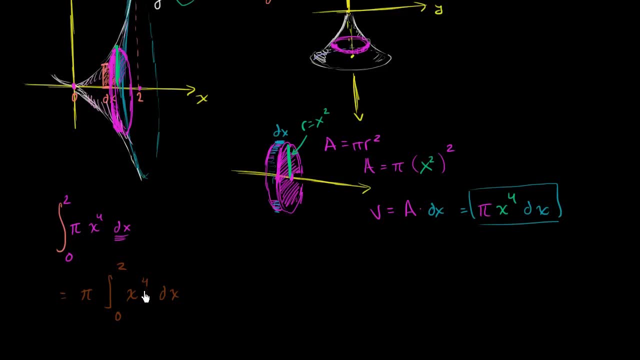 Now, the antiderivative of x to the fourth is x to the fifth over 5. So this is going to be equal to pi times x to the fifth over 5. And we're going to go from 0 to 2. So this is going to be equal to pi times this thing evaluated at 2. Let's see, 2 to the third is 8, 2 to the fourth is 16, 2 to the fifth is, let me actually just write it down, 2 to the fifth over 5 minus 0 to the fifth over 5.